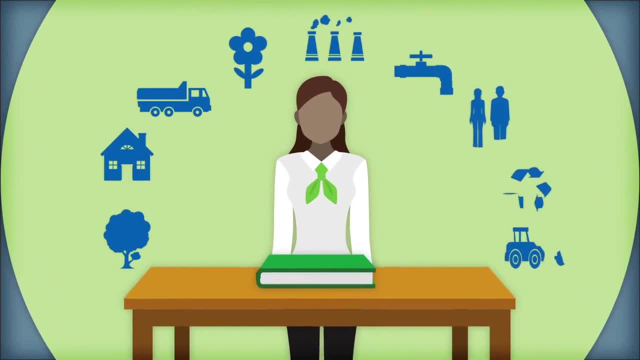 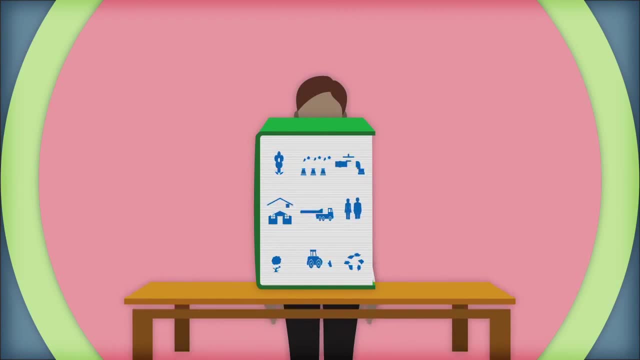 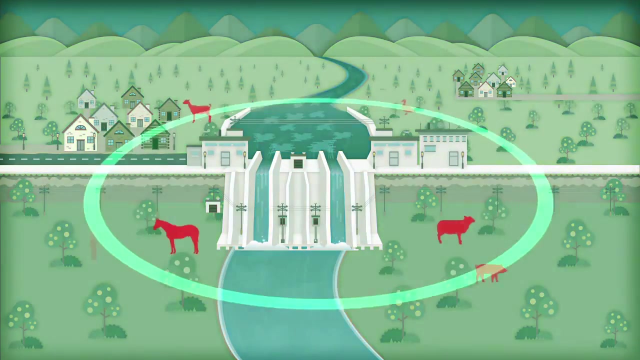 EIA can become overstretched and overburdened with irrelevant issues, require unnecessary efforts and cause problems With new development projects. there is a risk of generating site-specific impacts as well as impacts on the surrounding areas. The risks and impacts do not always decrease. 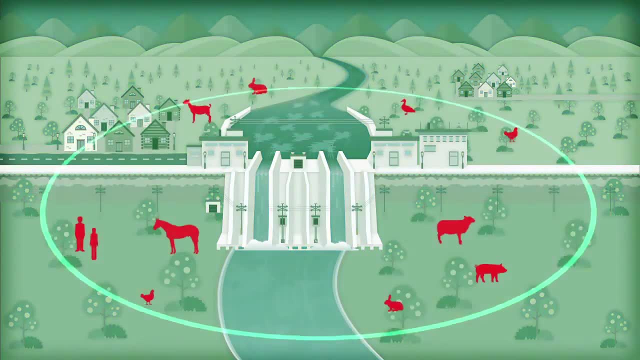 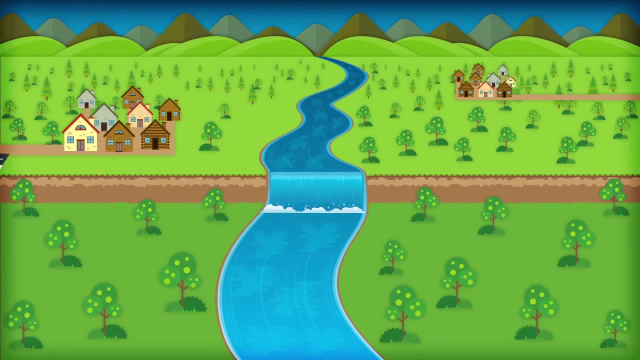 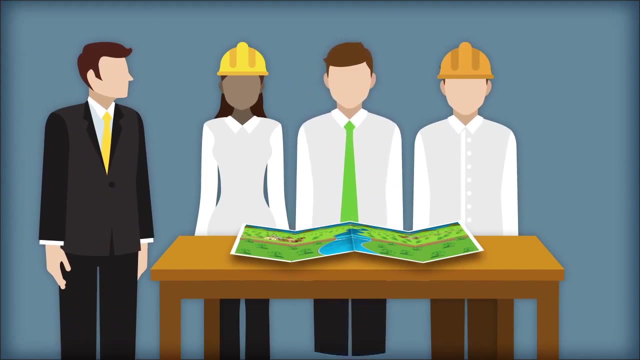 with an increase in distance from the project site. Some impacts are obvious, while others are not. The scoping phase should take place in the beginning of the EIA process and ideally include the participation of the reviewer- The participation of reviewers in this phase. 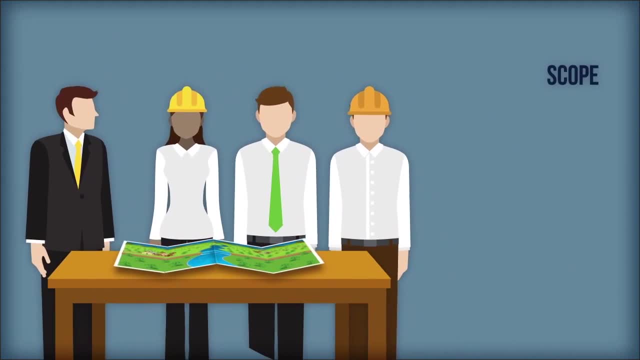 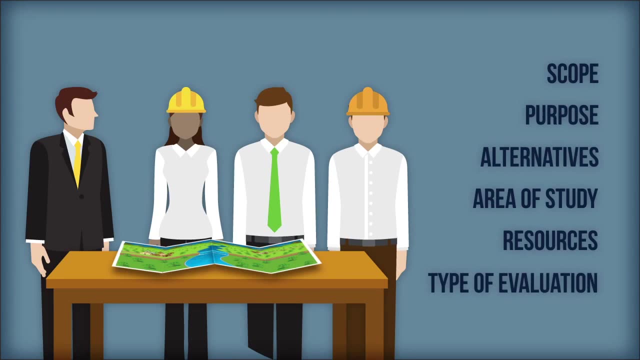 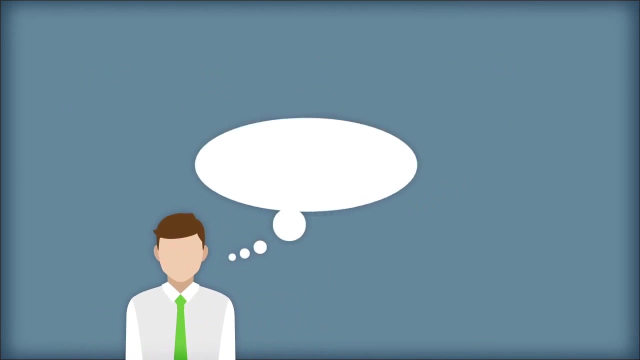 shapes the EIA process, including the scope, purpose, alternatives, area of study resources and the type of assessment. Unfortunately, scoping is often done before the reviewers are involved. In many cases, EIA reviewers are left to determine after the fact whether 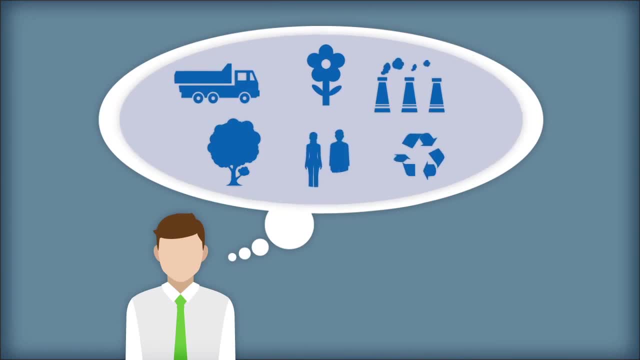 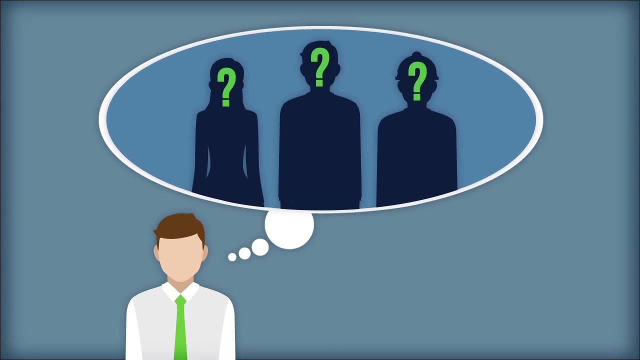 the scoping was done correctly, whether the correct number of topics and scenarios were contemplated, and whether all the information and perspectives were considered? Was there an opportunity to solicit views and comments from all the key stakeholders? Who was involved or consulted in the process of preparing the EIA, and in what way? 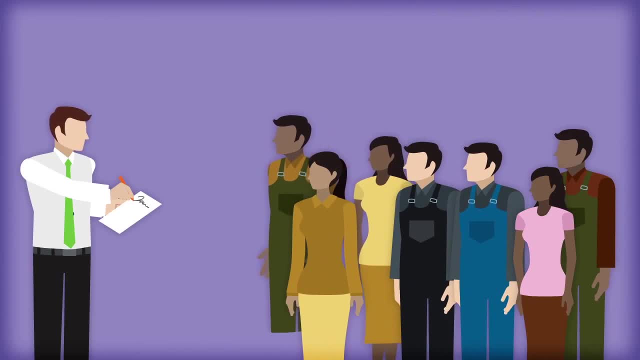 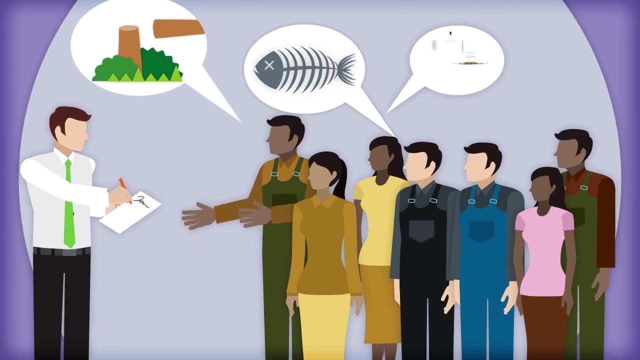 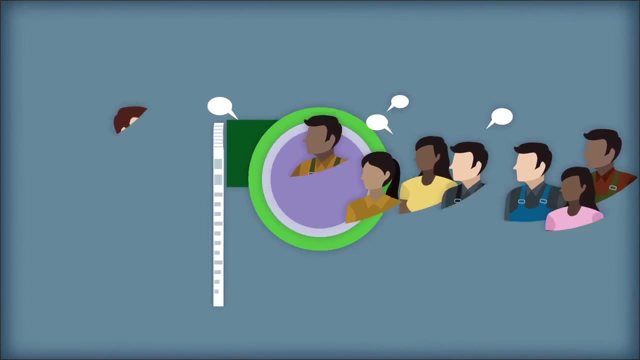 The benefits of communicating with and involving all stakeholders is important, especially for the EIA. During the EIA review, technical experts may overlook key information or areas of study that local citizens and communities can more easily identify due to their proximity to the potentially affected areas and greater stake in the outcome. Fortunately, when trying 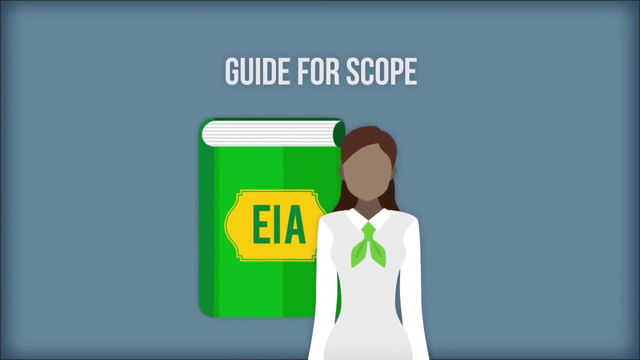 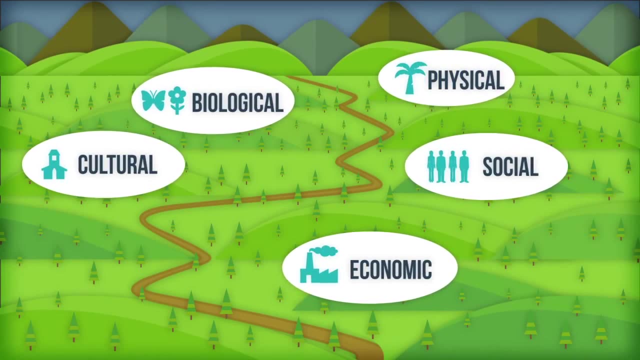 to assess or define the scope of an EIA. reviewers do not have to guess. Some helpful criteria for evaluating the adequacy of the scope of an EIA review is the following: Are potentially significant issues and interactions for natural and human environments indicated?